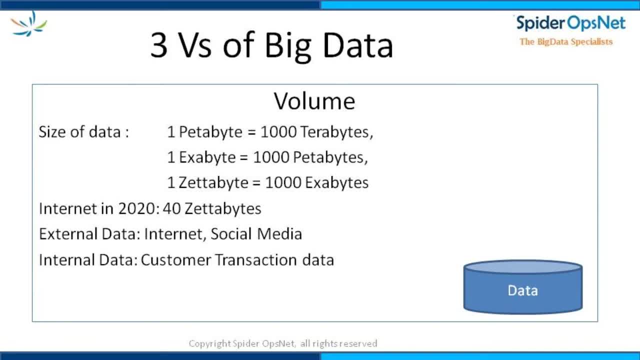 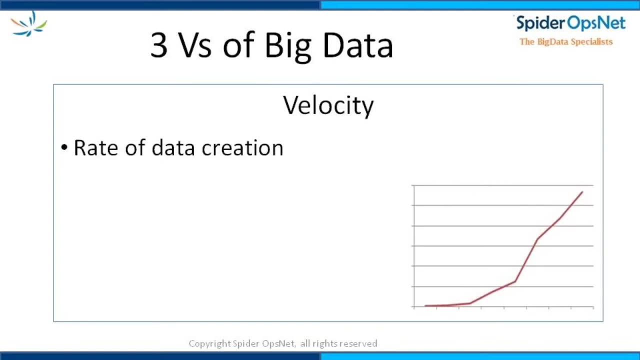 Internal data refers to the customer transaction data. How will organizations store and back up this much amount of data and process them efficiently? You need big data technology for that. Velocity refers to the rate at which the data is processed. Use of IOT sensors and multiple devices like tablets, smartphones and mobile devices is 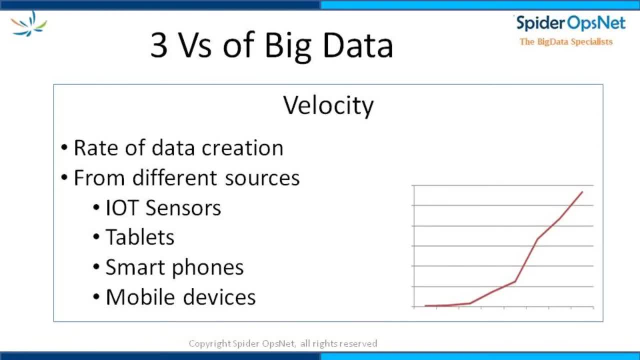 causing enormous increase in data velocity. A manufacturing unit may have thousands of sensors, with each sensor producing measurements every second or even multiple times per second. Hundreds of gigabytes of data may get generated every day and have thousands of megabytes of data, And it has to be processed immediately. 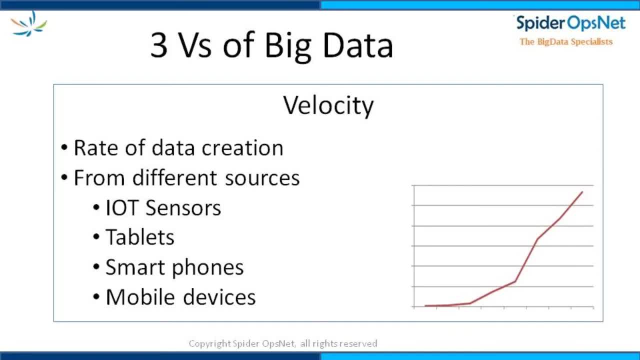 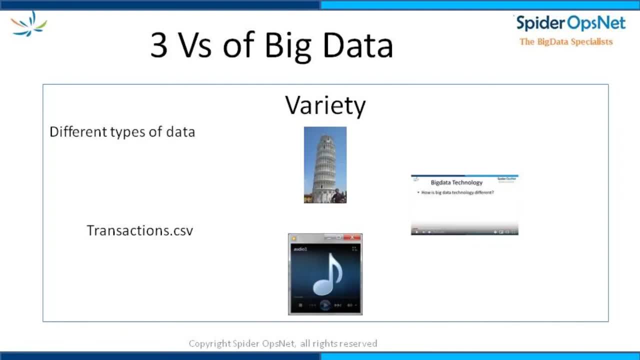 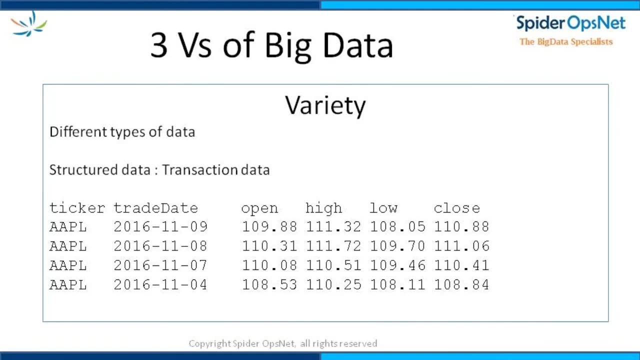 This is only possible with parallel and distributed processing of data using big data technology. Variety is another aspect of big data. Variety refers to multiple types of data that is being processed. An organization may have to process not only the structured transactional data, but also. 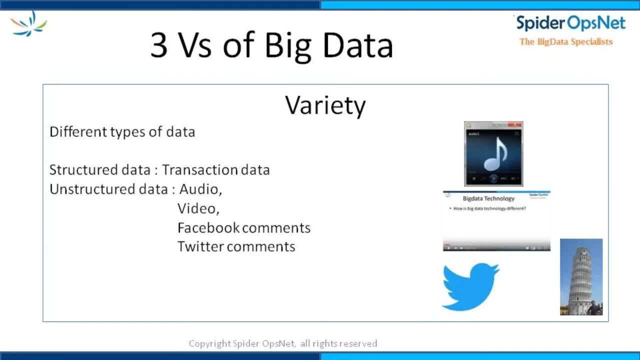 the unstructured data Like audio video etc. video, Facebook comments, Twitter comments etc. To do a competitor analysis. an R2O manufacturer did a trend analysis on the competitor's products using Twitter data to gauge the market reactions and positioned their models accordingly. 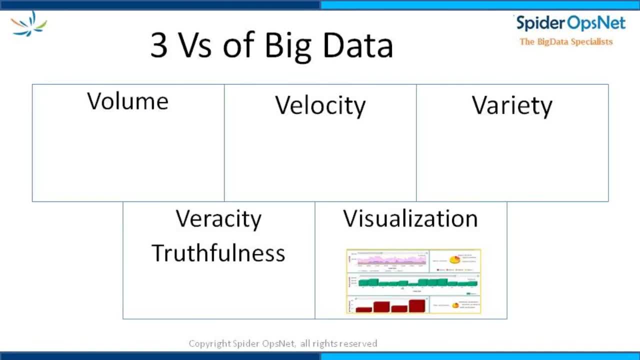 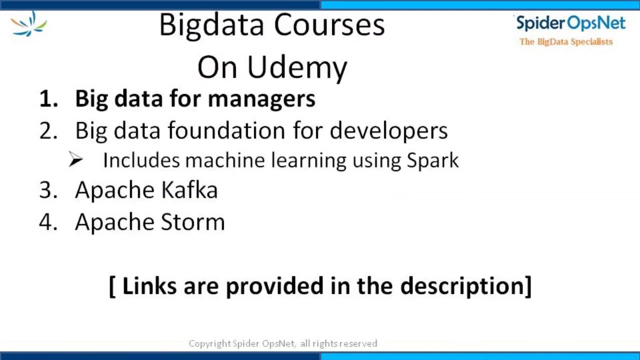 to get better market share. Apart from these three Vs, there are also some more Vs, like Veracity. that refers to the truthfulness of data. Visualization, that refers to the way data can be represented in a graphical format. If you want to learn more about Big Data, please subscribe to my courses on Udemy. 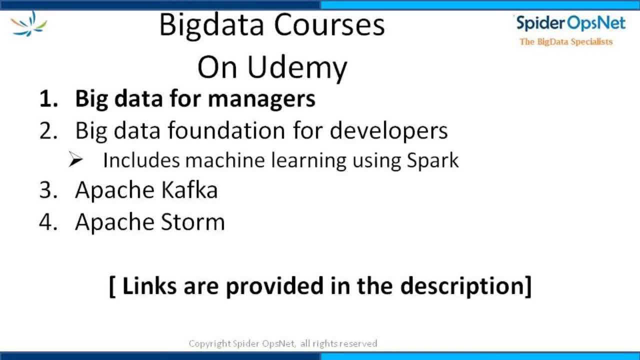